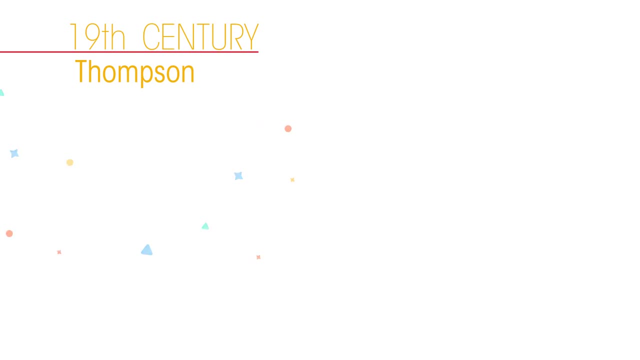 In the late 19th century, a man called Thomson expanded on Dalton's idea. He discovered the existence of electrons when making cathode ray beams interact with electric and magnetic fields. He determined that the cathode rays consisted of a beam of negatively charged 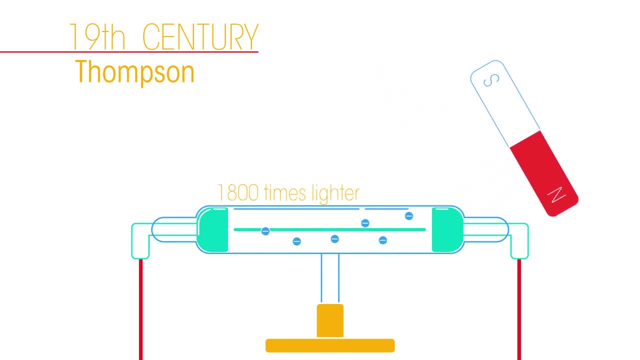 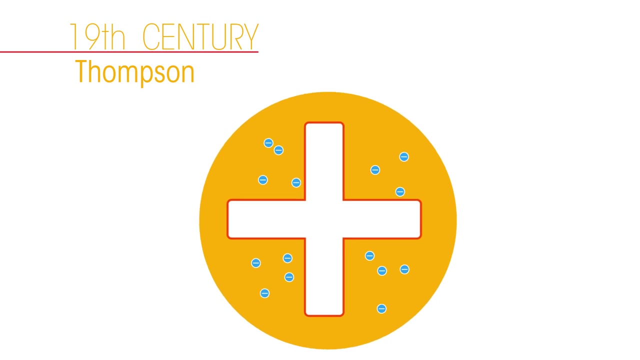 particles that were 1800 times lighter than the lightest known atom, hydrogen. His discovery showed that atoms are made up of even smaller particles. He proposed the plum pudding model of the atom, whereby the atom is a positively charged sphere within which electrons swim. 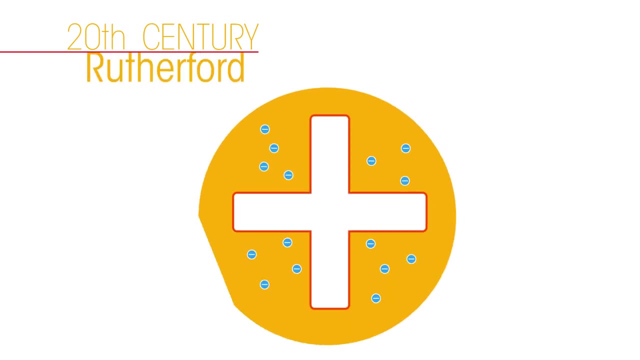 In the early 20th century, experiments designed by a man called Rutherford indicated that the plum pudding model was not entirely correct. Two of his assistants, called Geiger and Muller, carried out the study. They used alpha particles, which are very tiny positively charged particles. They aimed a beam of alpha particles at very 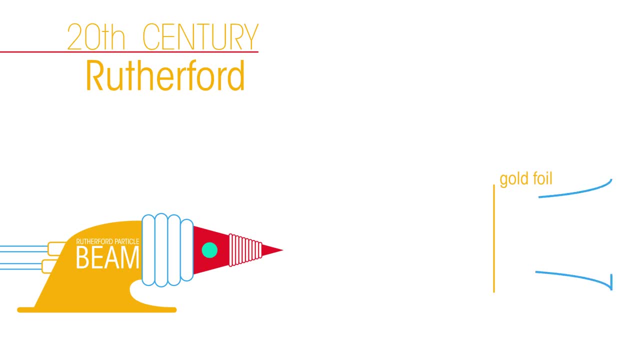 thin gold foil. If the alpha particles got through the foil it would be detected by a sensor. Translating the theory to the Helmholtz problem, the answer is no, Assuming Thomson's plum pudding model was correct, they expected all alpha particles would pass through the gold foil and be detected on the 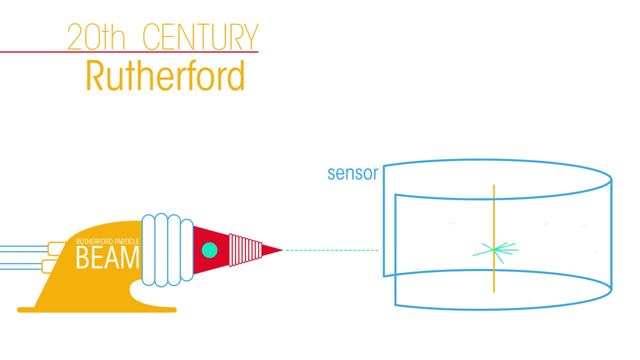 other side. However, while some did show this behavior, others emerged at unexpected angles and some even deflected back to the alpha particle emitter, never passing through the foil. They concluded that the alpha particles were being repelled and deflected by the tiny concentrations. 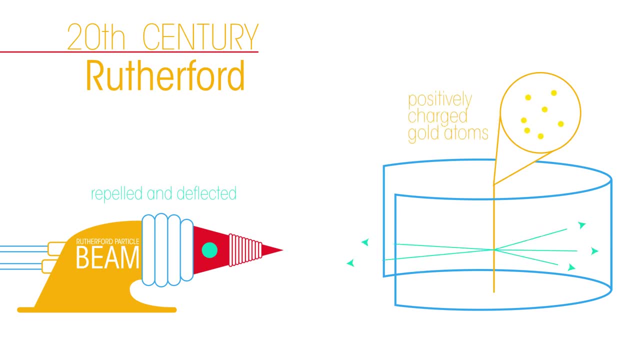 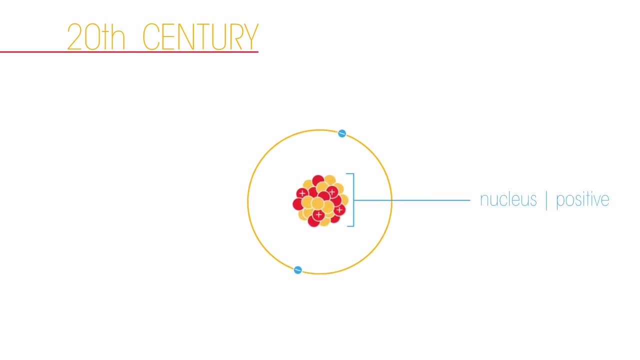 of positively charged subatomic particles within the gold atoms which made up the gold foil. Since his discovery, atoms have been described as having a central nucleus of positive charge which is orbited by negatively charged electrons. This is known as the nuclear model of the atom. 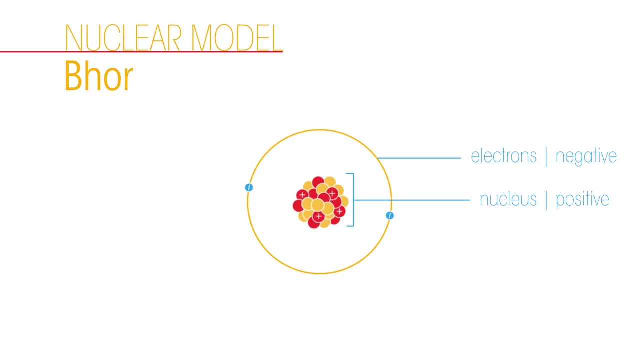 Bohr developed Rutherford's nuclear atom model further. He concluded from his own experiments that electrons occupy specific orbits or shells around the nucleus. In other words, electrons orbit the nucleus similar to how planets orbit the sun. However, electrons can also orbit the nucleus in the same way. They can also orbit the nucleus in the same way.